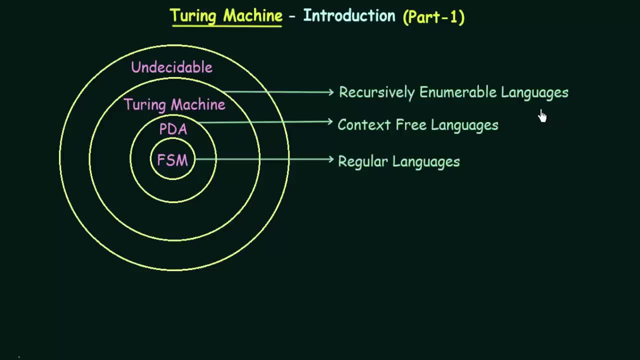 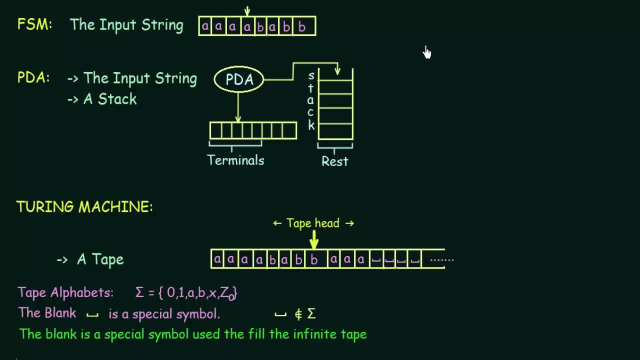 which we will be discussing in detail as we proceed further in this module of Turing machine. Now let us see what were the data structures that we had in finite state machines and push-down automata, And let us see what is the kind of data structure that we will have in Turing machines. 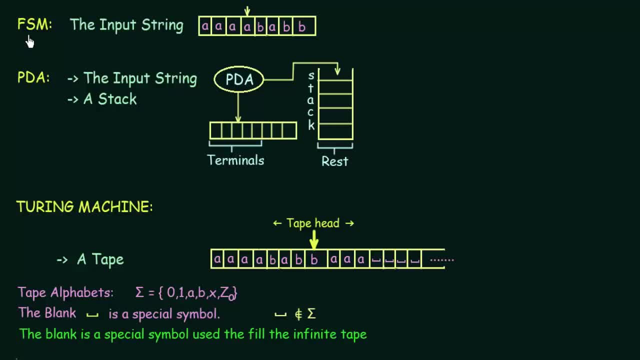 So, if you remember, in case of our finite state machines which accepted the regular languages, the data structure that we had was only the input string. We just had an input string and we had a control which can move only to one direction and that is forward. 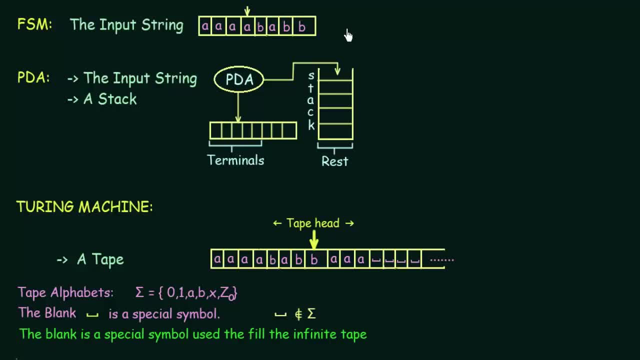 So we saw the finite state machines and we saw that they had a very limited power And also a very limited memory. and the class of languages accepted by finite state machines are the regular languages, and we already saw what are those regular languages. And coming to push-down automata: in push-down automata, the data structure that we had was the input string. 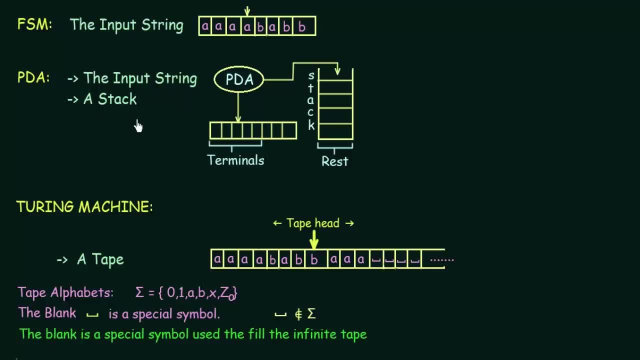 and apart from the input string, we had a stack. So what made the push-down automata different from finite state machine was the presence of a stack. So because of the presence of this stack, we saw that the push-down automata was more powerful than finite state machines. 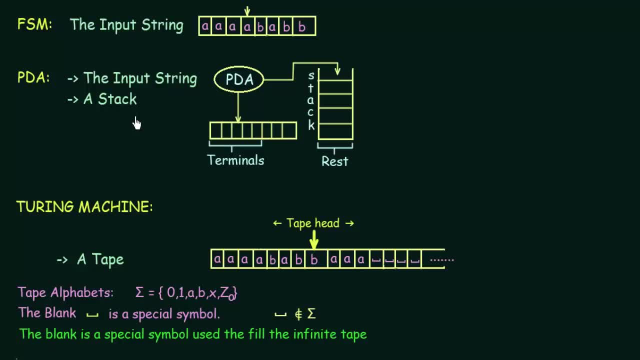 and then the class of languages that they accept, which is known as the context-free languages, are a higher class of languages as compared to regular languages. So this is the diagram which represents that we had the input string and also the stack which added more power to the push-down automata, making it different from the finite state machines. 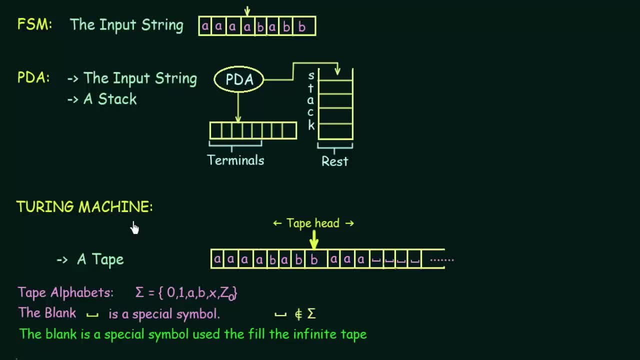 Now coming down, we have the Turing machines, which we are going to discuss. We are going to discuss in this lecture, And in Turing machine, the data structure that we have is something known as a tape. So a tape is something that looks like this, as it is shown in this diagram: 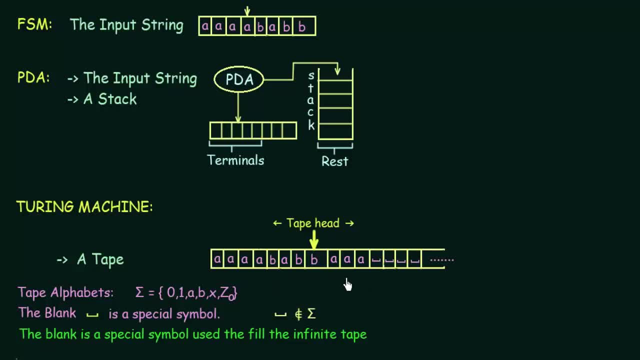 So we see that the tape is a sequence of infinite symbols. It is an infinite sequence and over here we have something known as a tape head. So the tape head is positioned on the symbol and the current control is present. And then the tape head, it can either move one step to the left or one step to the right. 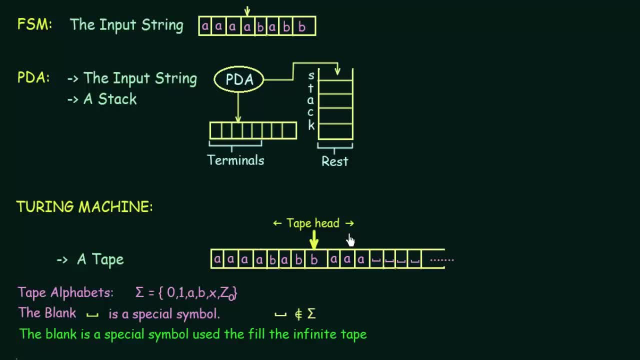 depending on the kind of computation that we have. And then here we have the input symbols and, as I told you, this is an infinite sequence. So the input symbols that we have, they are filled into these cells and then the remaining cells, instead of leaving them just blank. 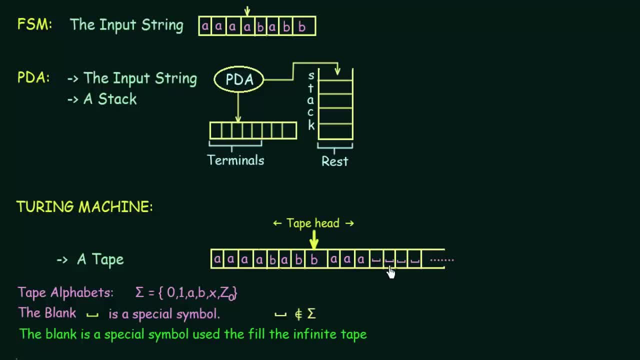 we fill them with a special kind of symbol That is known as the blank symbol And if you see, here we have the tape alphabets, which is represented by sigma. You know, sigma is used to represent the input symbols. We have been studying this from the beginning of this lecture series. 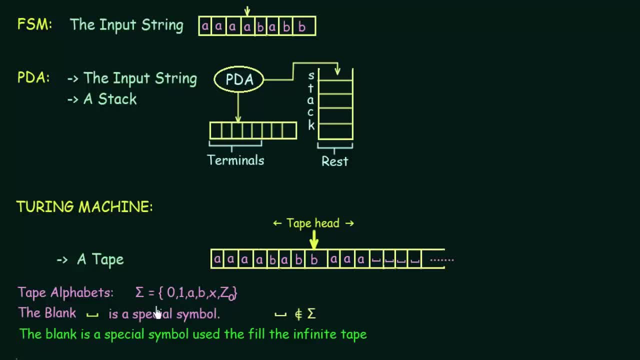 And the tape alphabets. it can contain 0,, 1, A, B or any kind of symbols like this. And then, as I told you, the blank symbol is a special symbol And something you need to note is that the blank symbol- it does not belong to sigma. 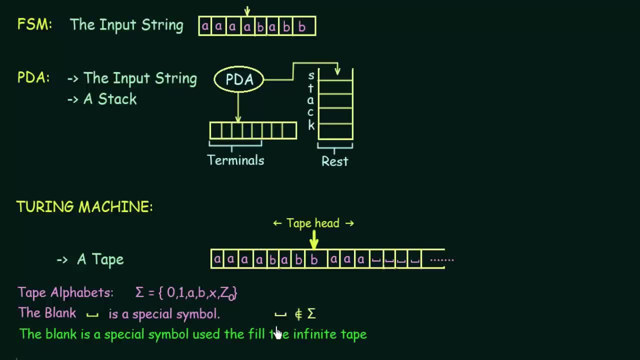 That means the blank symbol is not a part of the tape alphabets, or it is not a part of the input symbol. But what is it? It is just a special symbol that is used to fill the infinite tape. So, as we are having an infinite tape, 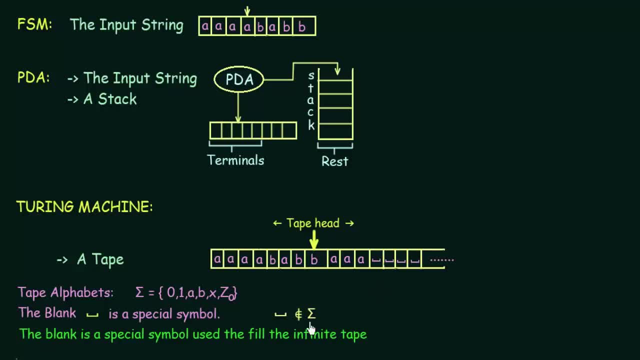 the blank or the empty cells are filled with this special symbol, known as the blank symbol, represented by this. So this is the basic data structure that we have in our Turing machine. So the main thing that you need to remember is that the tape is an infinite sequence. 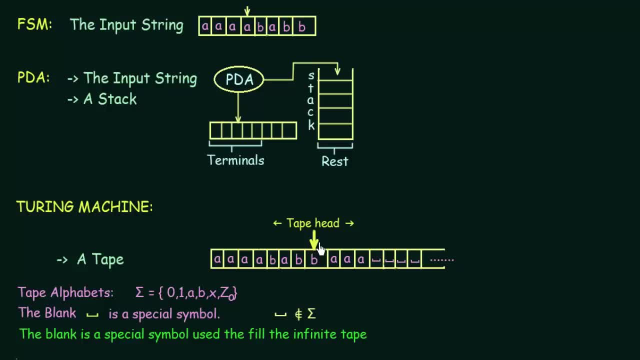 And then the tape head is the position where the current control is present, And then the empty cells are filled in by a special symbol known as the blank symbol. Now let us look at the initial configuration of a Turing machine. So if we have a Turing machine, 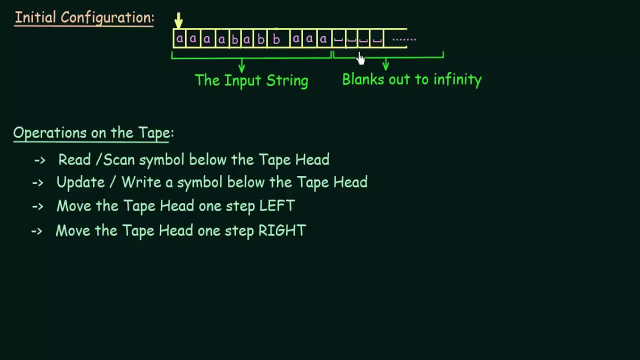 the initial configuration of the tape, it looks something like this. So here, as I told you, we have the input strings represented by these symbols over here, And then the empty cells. it is filled by these symbols, known as the blank symbol. 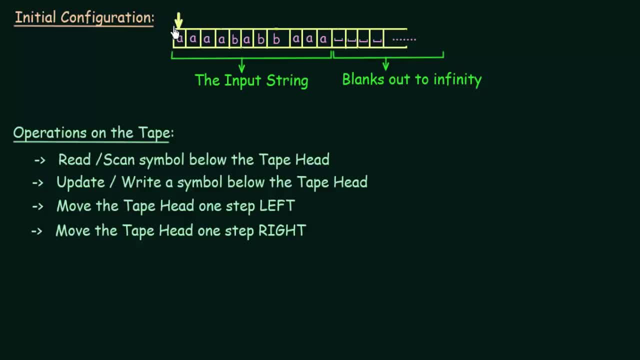 So it blanks out to infinity. And then we have the tape head, which is positioned on the leftmost end, at the starting, And now let us see what are the operations that we can have on the tape. So these are the operations that we can have on our tape.